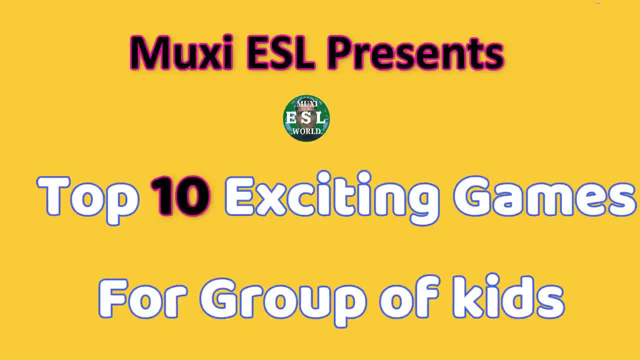 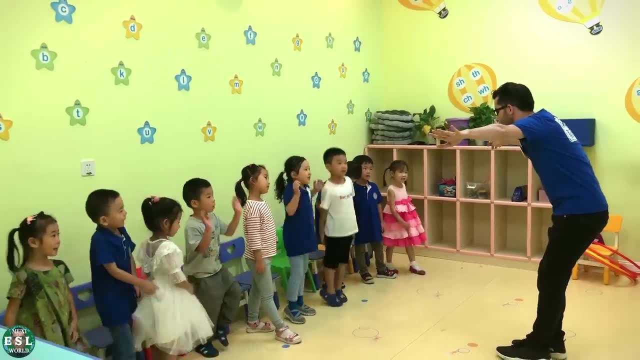 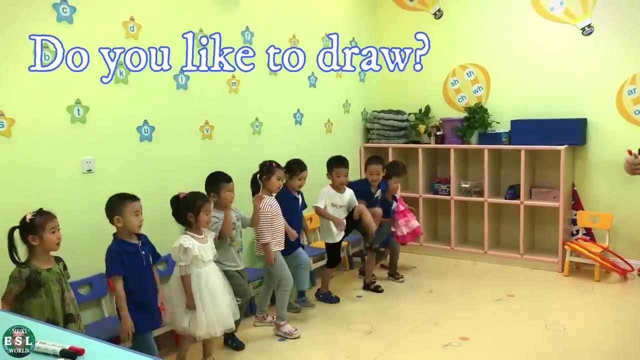 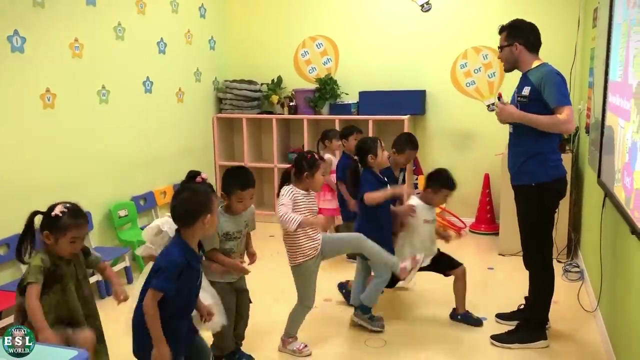 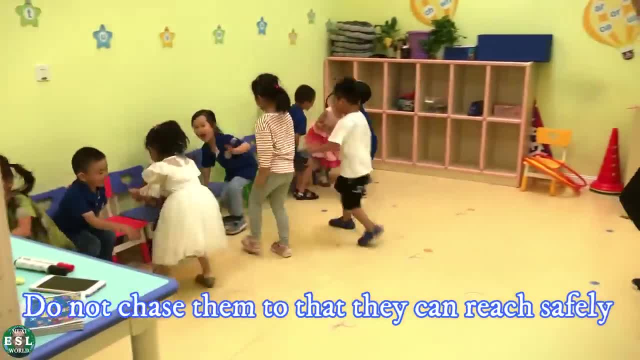 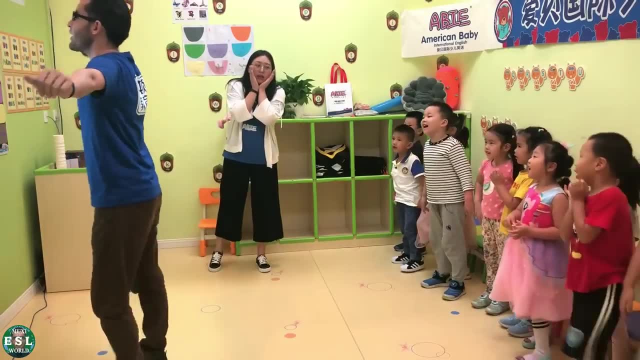 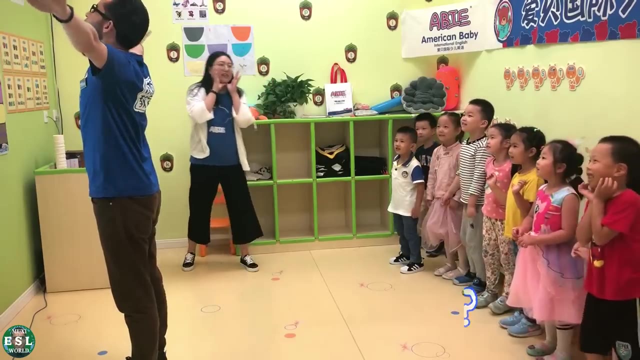 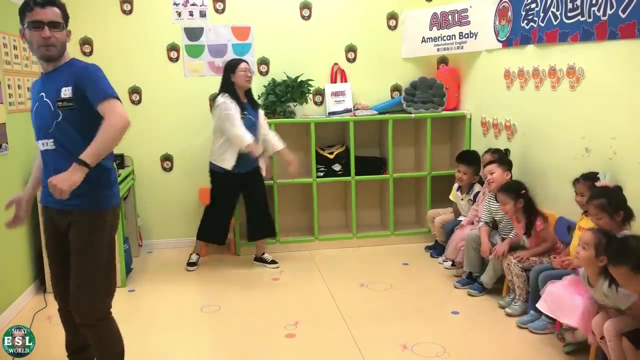 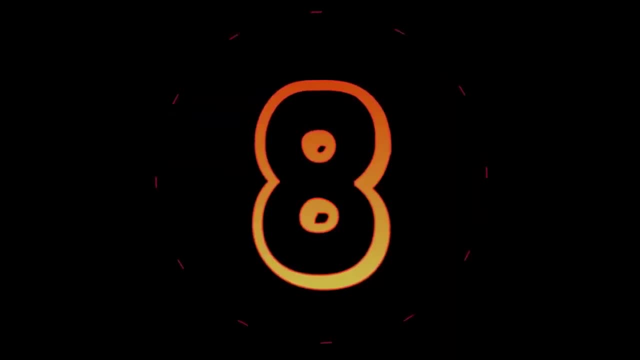 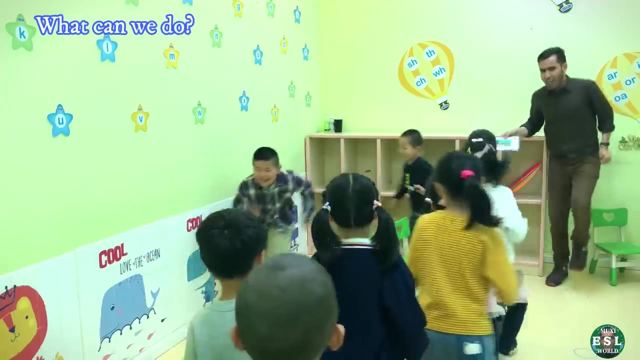 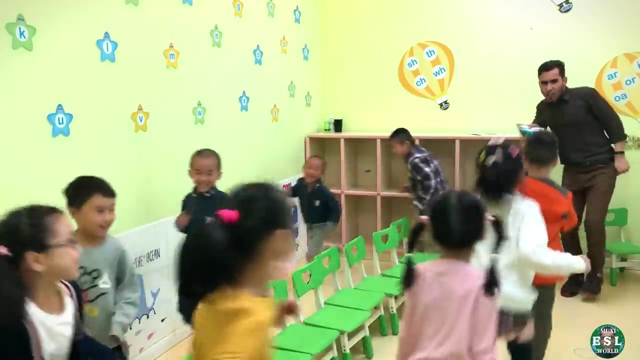 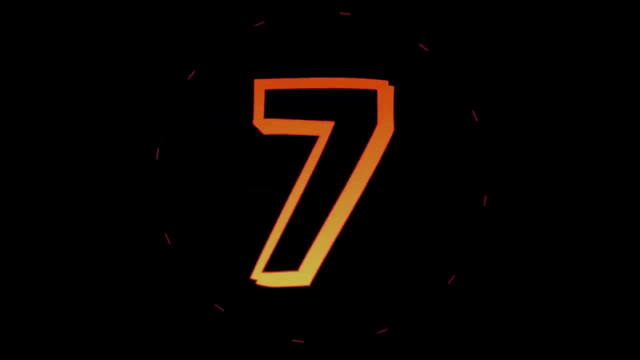 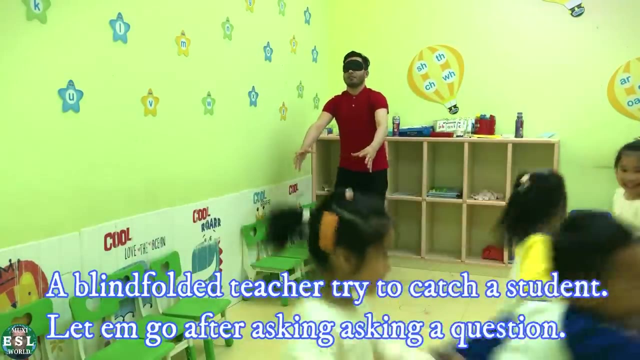 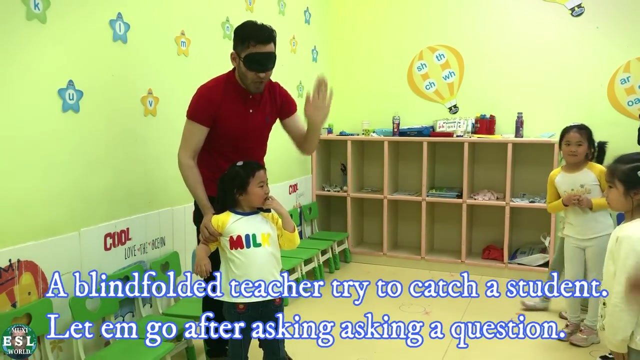 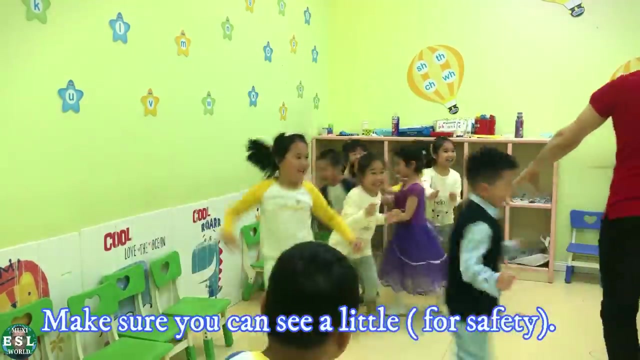 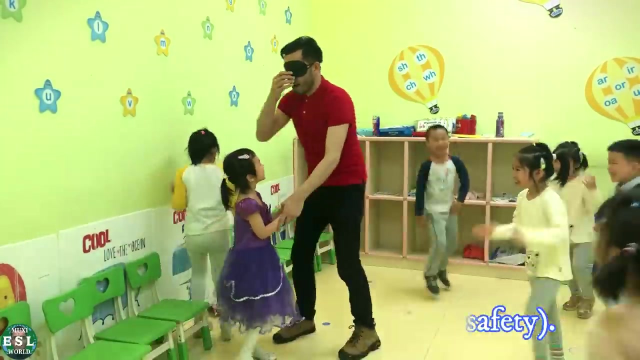 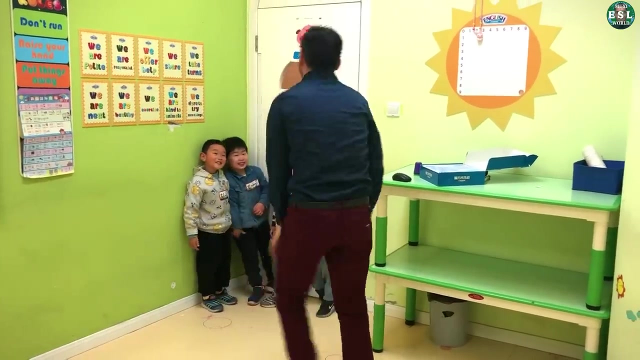 Never go later. Say it Bells ringing. I got it. Everybody stop, Everybody stop. Who are you? I am the gym teacher. Ok, ready, go. Ok, who are you? Say it's a pig, It's a pig. 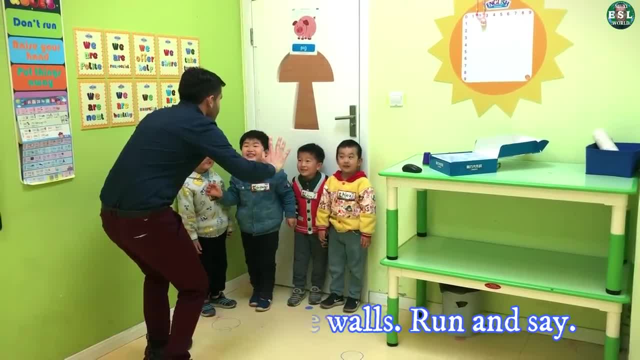 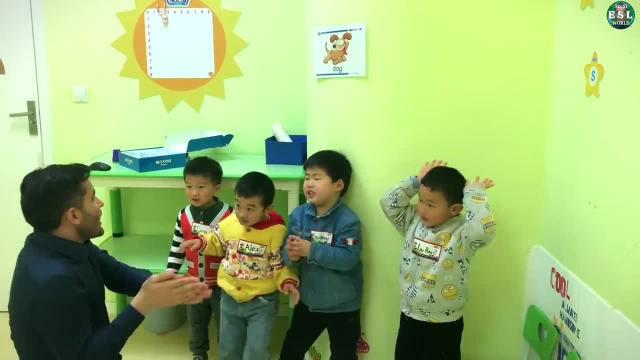 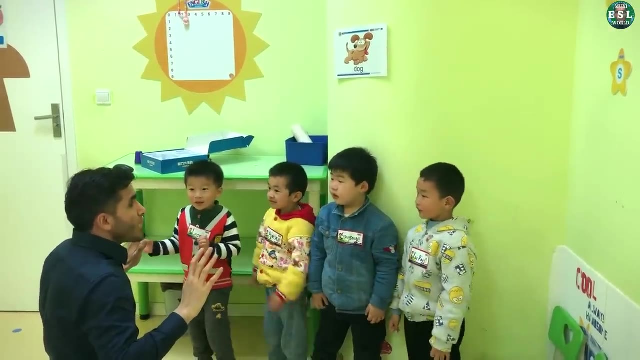 It's a pig, Now it's a dog. It's a dog. Say it's a dog, It's a dog. Everybody say woof, woof, Woof, woof. Where is the cat Cat? Now everybody say it's a cat. 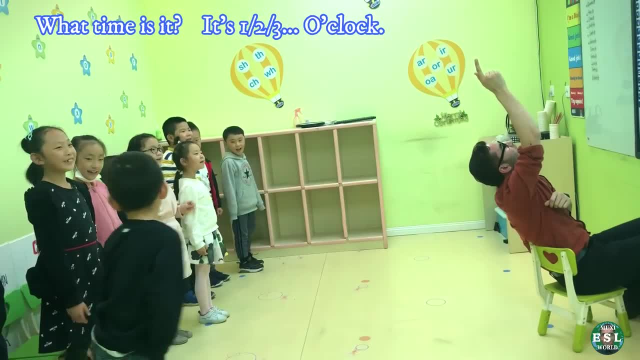 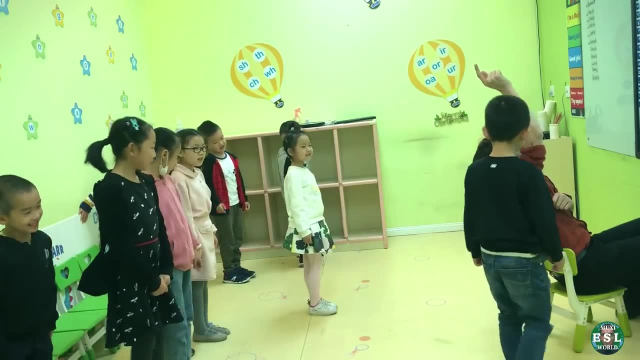 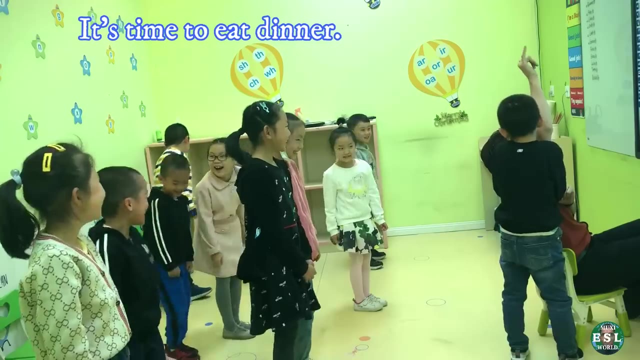 It's one o'clock. What time is it? It's two o'clock. What time is it? It's three o'clock. What time is it? It's four o'clock. What time is it? It's five o'clock. What time is it? 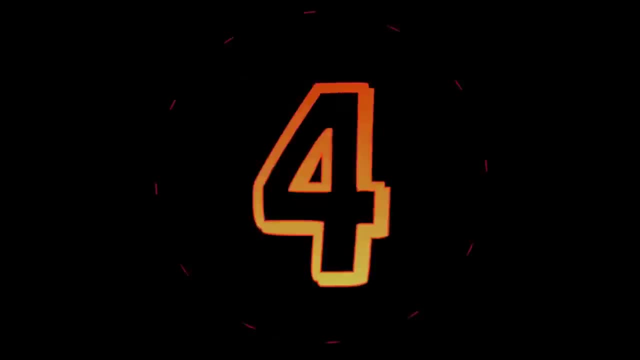 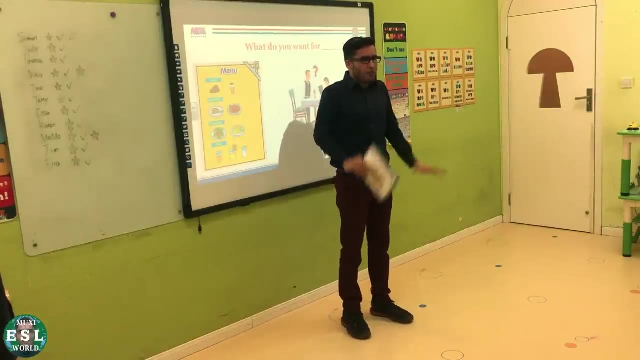 It's six o'clock. What time is it? It's time to eat. When Mushy covers his eyes, he's gonna move slowly. When Mushy sees you, everybody will freeze, Everybody ready. What do you want for the main dish? 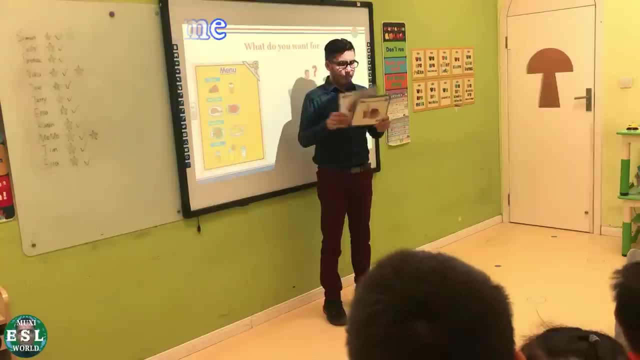 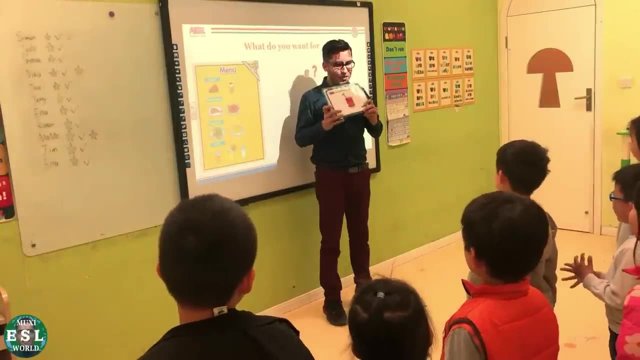 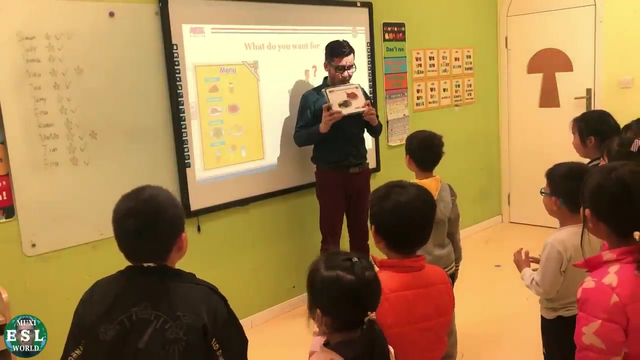 I want cheese and peas. What do you want for vegetables? I want salad, please. What do you want to drink? I want green tea, please. What do you want for the main dish? I want peanut, please. Mushy is hungry. 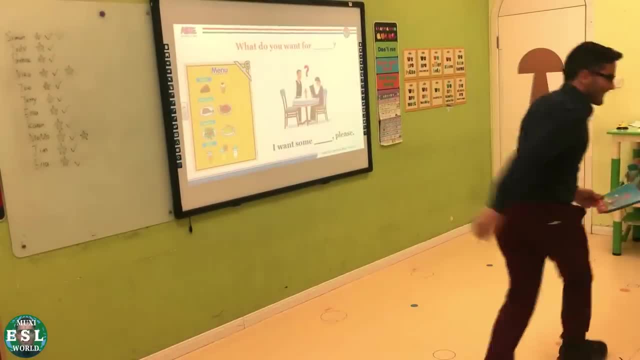 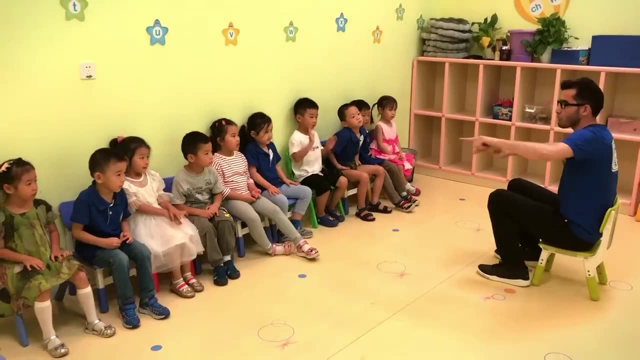 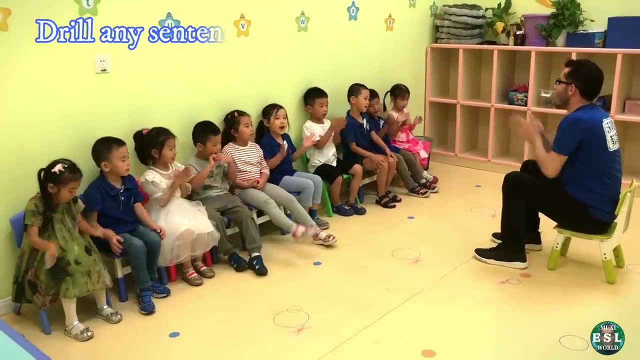 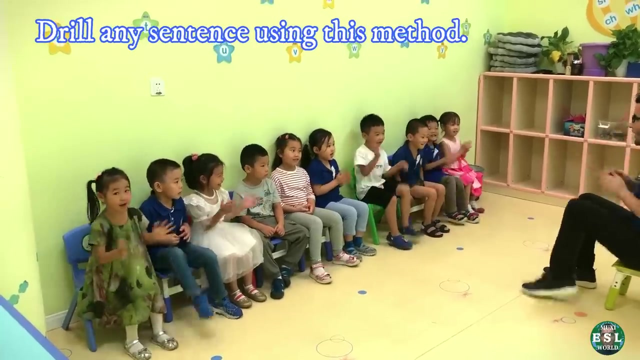 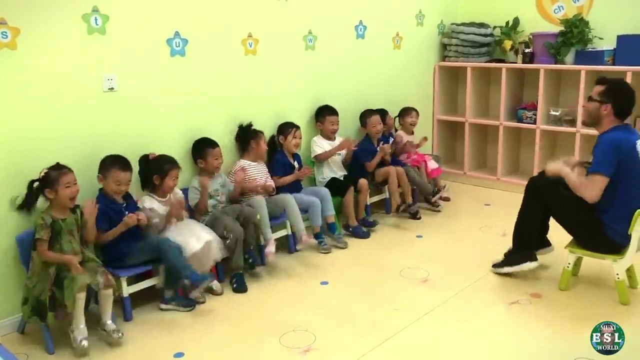 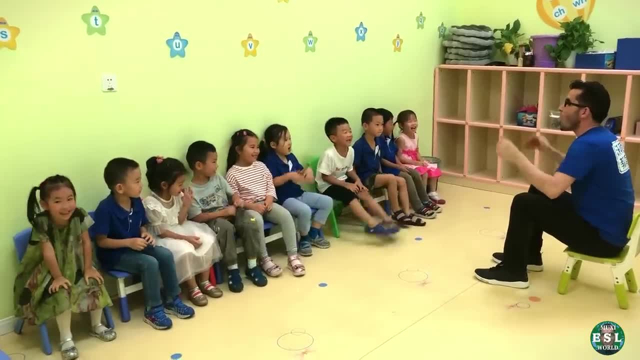 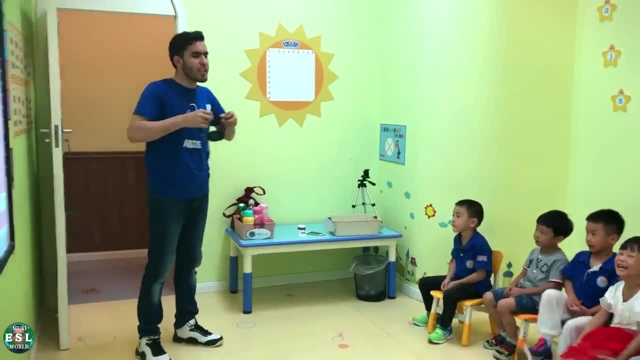 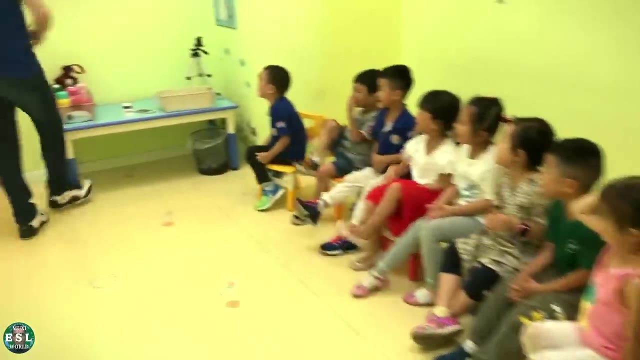 Draw and color One more time. Draw and color. That was it, Okay, guys. so we are going to practice. what do you see with right? I'm gonna blindfold myself like that. Keep chanting. say: What do you see with? 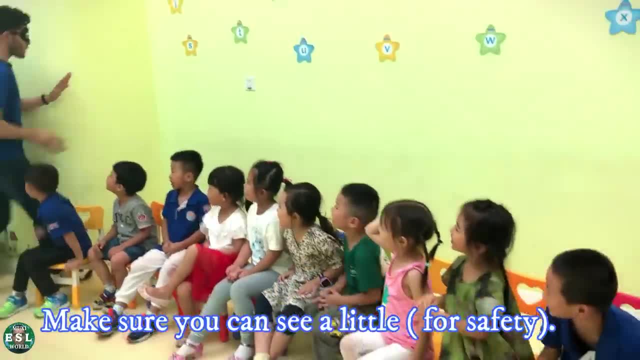 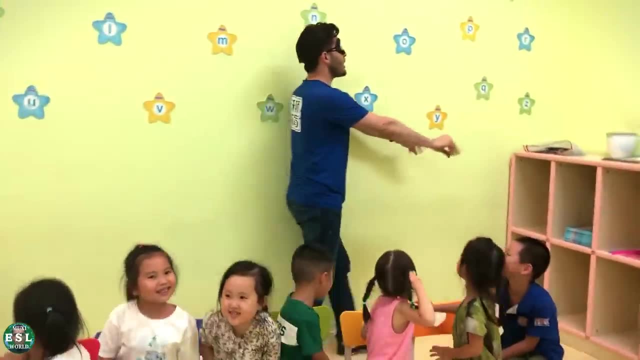 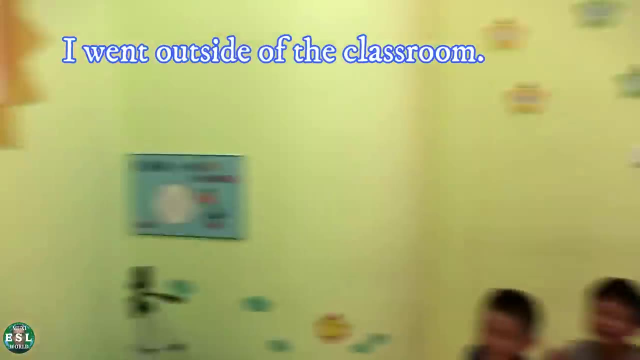 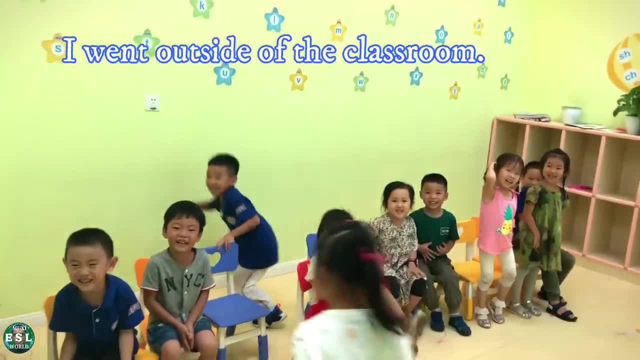 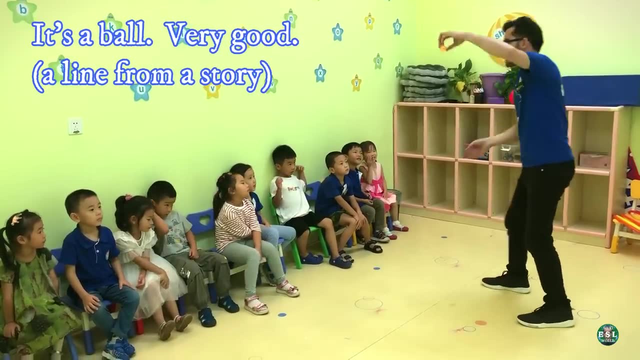 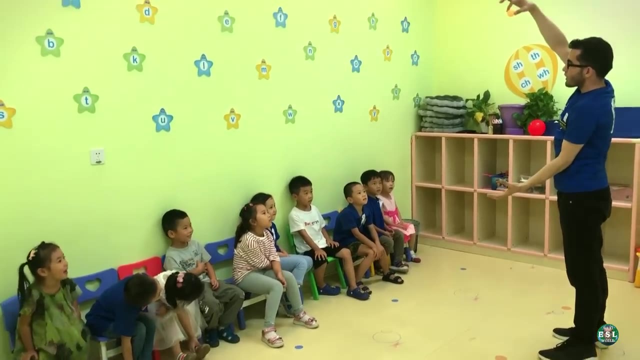 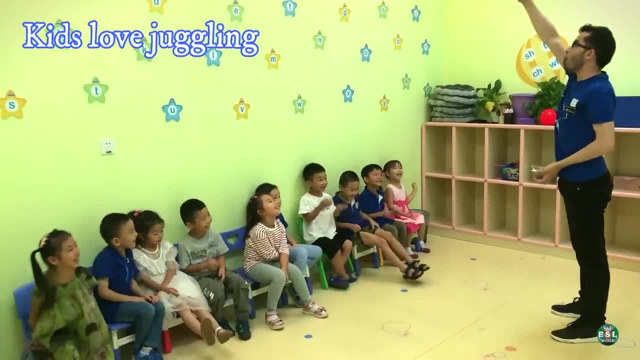 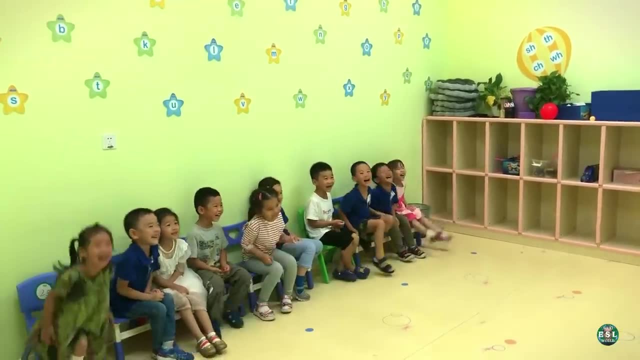 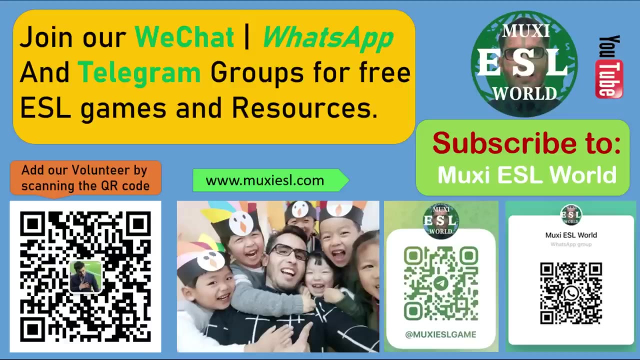 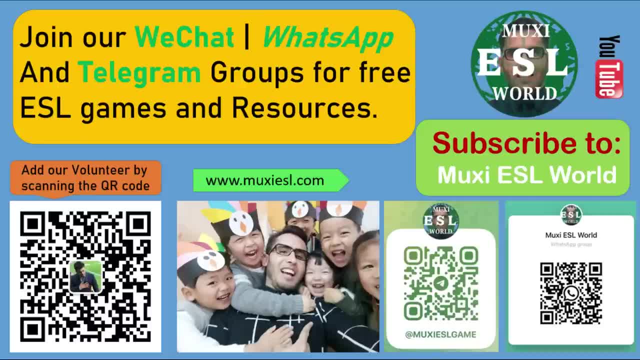 What do you see with? What do you see with?